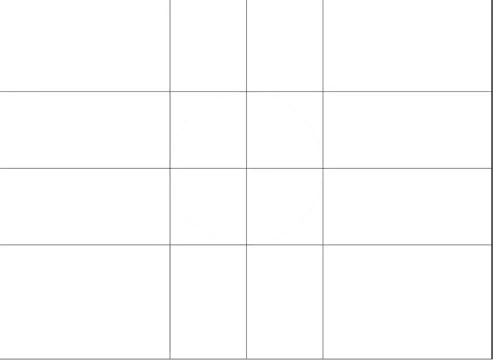 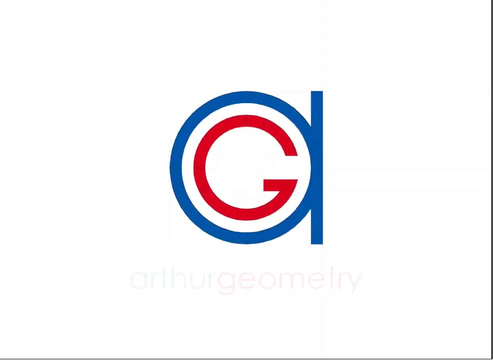 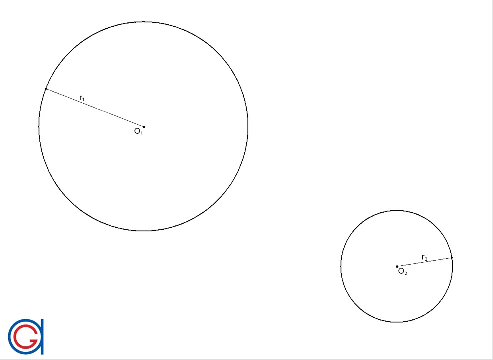 Hello, today we are going to learn how to draw the two internal tangent lines of two given circles. Here you can see two given circles with center points O1 and radius R1 and with center points O2 and radius R2.. So the first step is to join the center points O1 to O2.. 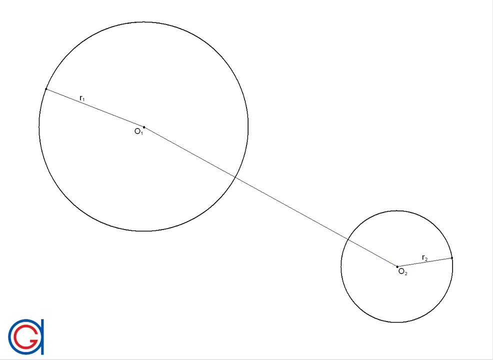 The next step is to work out the perpendicular bisector of the line O1- O2.. So to do this, we set our compass slightly longer than half the distance and we describe an arc to the right, as can be seen here And now, with the same radius and setting our compass on point O2. 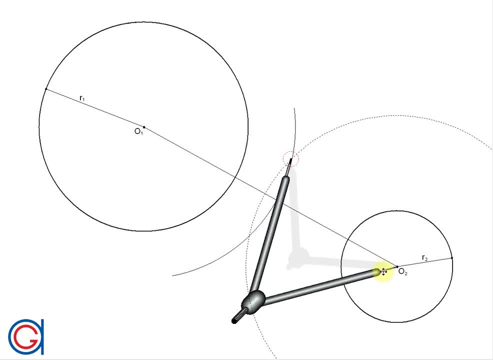 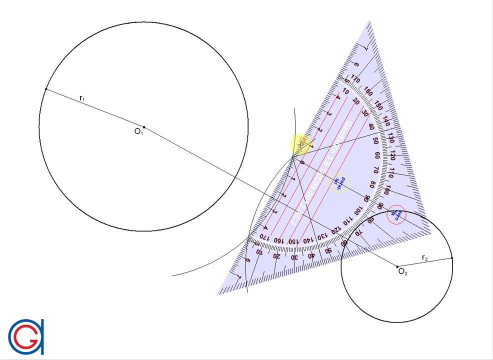 we describe another arc to the left, cutting our previously drawn arc at two points, and now, where these two arcs intersect, we're going to join them using a line and where it cuts the line, 0, 1, 0, 2 will be the midpoint M. 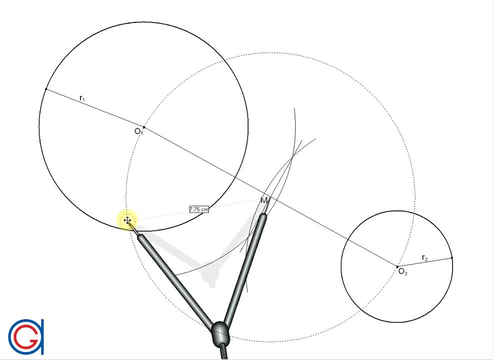 okay. so now, setting our compass on M, and with the radius M 0- 1, we're going to draw a circle which passes through both origins, 0, 1 and 0- 2, as can be seen here. so next we are going to add radiuses R 1 to radius R 2, but before we do this, we are going 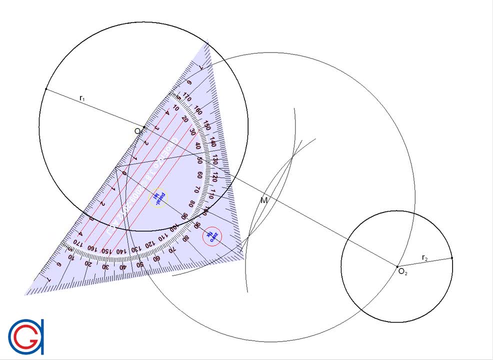 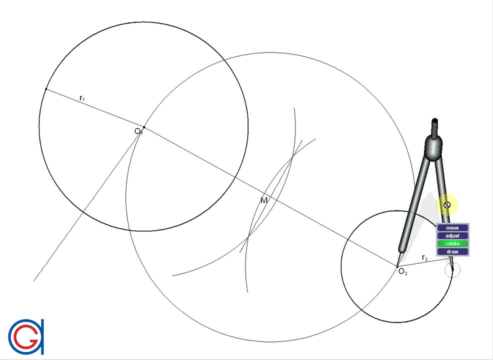 to draw a ray from point 0: 1 at any angle, and this ray must be longer than the addition of these two radius, as can be seen here. so now, setting our compass to the length of radius R 2, we're going to draw a circle which passes through both origins, 0, 1 and 0: 2, as can be seen here. 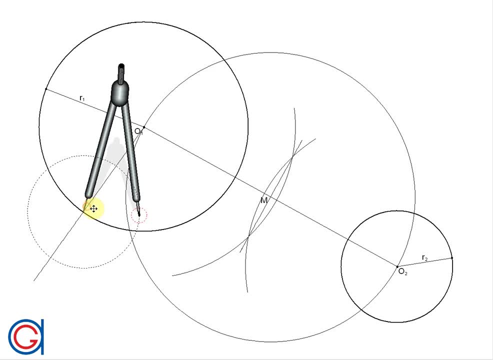 to the intersection point of the ray with the circle, as can be seen here, and where it cuts the ray is going to be our new radius R 1 plus R 2. so now setting our compass on 0, 1 and radius R 1 plus R 2. 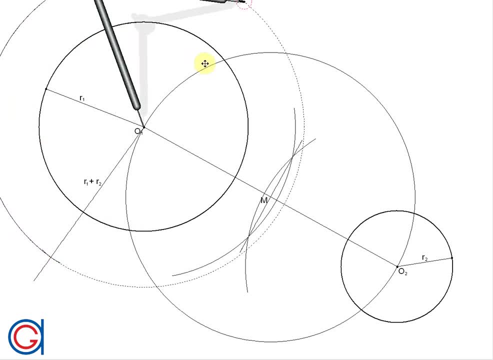 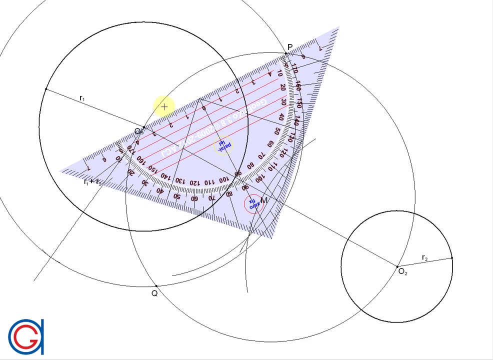 we will draw another external circle, as shown here. this new circle intersects with the previously drawn circle in the middle at two points, which we will call P and Q. so the next step is to join points 0, 1 with P, and where it cuts the internal circle will be our first. 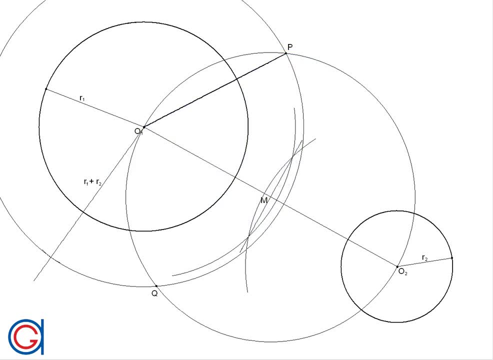 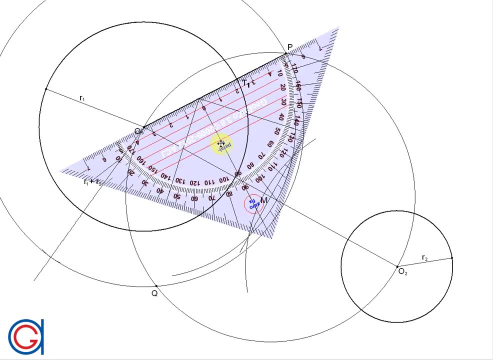 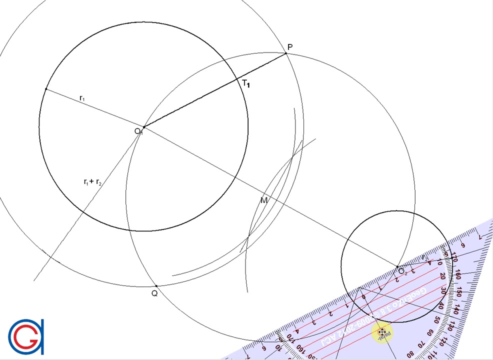 internal tangent point, which we will call T 1, and now we will draw a parallel line from this line, from point 0, 2, but in the other direction, obtaining our second internal tangent point, T 2, as seen here. we can see that the center of the solar center, 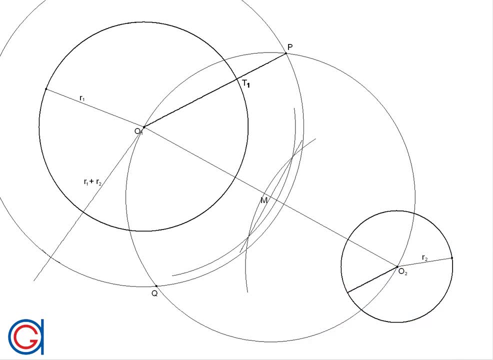 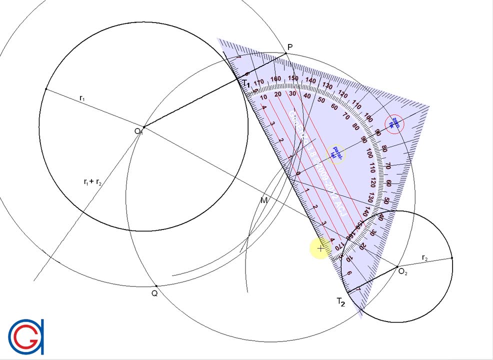 passes through the GORDON´s curve. whereol touch the outside of the circle, as shown here & now, is tanta T2, & now we are going to draw an internal tangent line is passing through points T 1 and T 2, & now we will repeat this process on the other side. 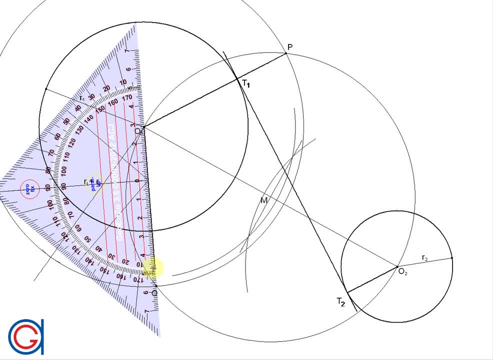 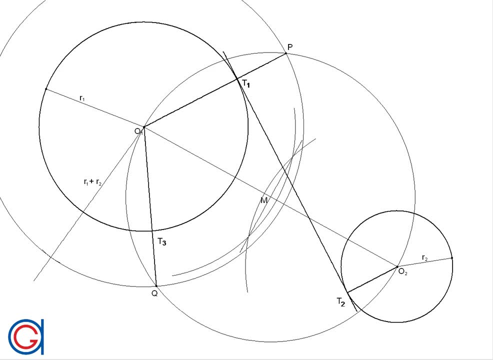 V"0, 1, 2, point Q and where it passes through the internal circle will be our tangent point 3. and now we're going to draw a parallel line to this from O2 in the other direction until it touches the outside of our smaller given circle. 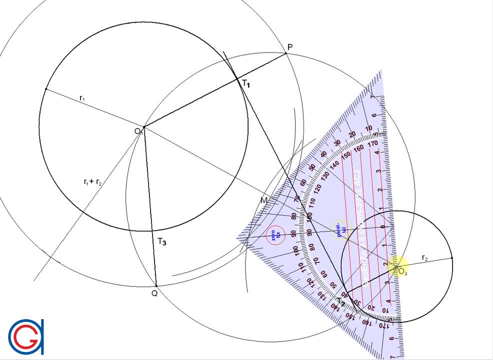 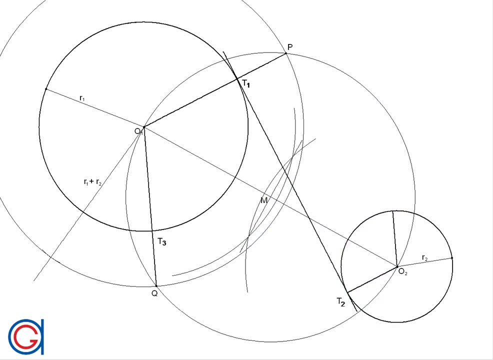 obtaining tangent point 4. so now we're going to join tangent point 3 to tangent point 4, our second internal tangent line, as can be seen here. okay, so we're going to check for perpendicularity and mark the angles with the symbols of parallelism. 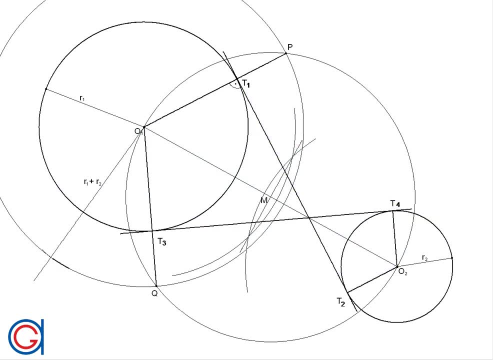 so you can see everything is parallel. ok, we can see there we go. so you can see everything is parallel. so we can show that there are no angles and everything have 90 degree angles. We can check with our 90 degree set square, as you can see here. Okay, so I hope this video has helped you.